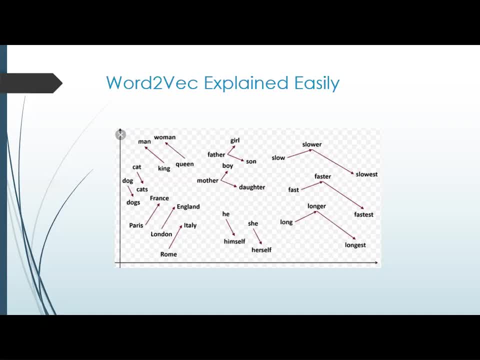 Now let us go ahead and start. So let's go ahead with this particular topic that is, Word2Vec. Now, you know that we usually convert the sentences, You know, whenever we are trying to apply natural language processing and when we are doing some spam classifier for each and every text. 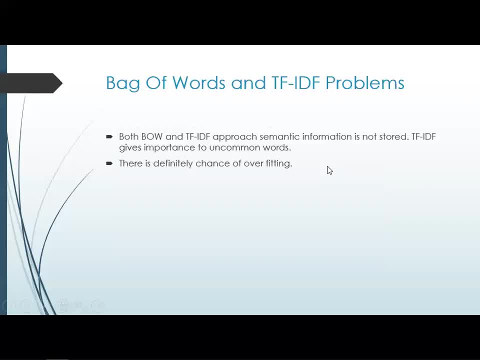 we usually convert them with the help of. we convert them into vectors with the help of bag of words and TFIDF. If you don't know about this particular stuff, guys, please make sure that you watch my complete playlist of NLP. 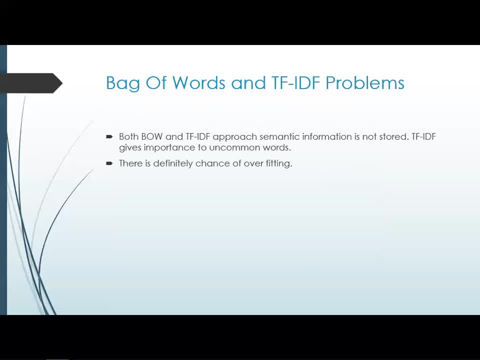 The link is given in the description. It would be very, very helpful for you. Now there are some problems with the help of bag of words and TFIDF, So let us understand what are basically the problems. Now suppose I have a sentences like I am going outside and I'm eating, for this kind of sentences are there with the help of bag of words. 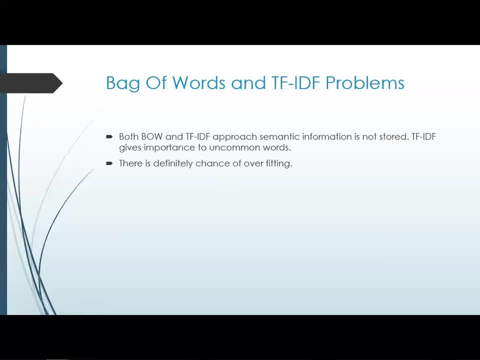 What we do is the bag of words model right. What we do is that wherever this particular word exists, you know, we actually make it as one and remaining word We make it as zero. Basically, We apply some kind of formulas based on histogram, number of count of words. most frequently what we create- a matrix, a lot of information. 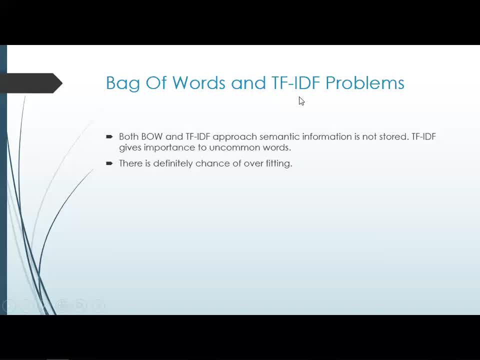 Similarly, in the case of TFIDF, which is also called as term frequency and inverse document frequency, We apply some log formulas to it and we assign some values, some integer values, to the most uncommon word, And we try to give importance to uncommon words. 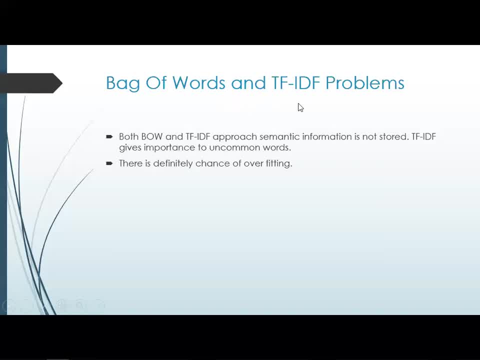 Now there are some problems with respect to bag of words and TFIDF. One of the problem is that they do not actually. in both Bag of words and TFIDF, semantic information is not stored. Now, what is semantic information? 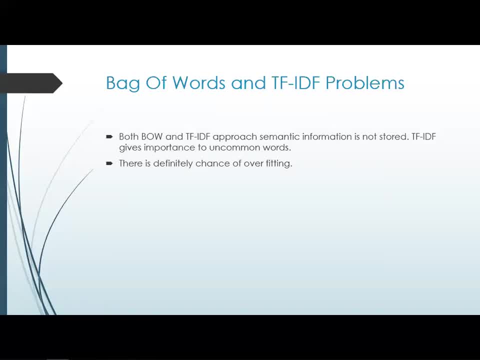 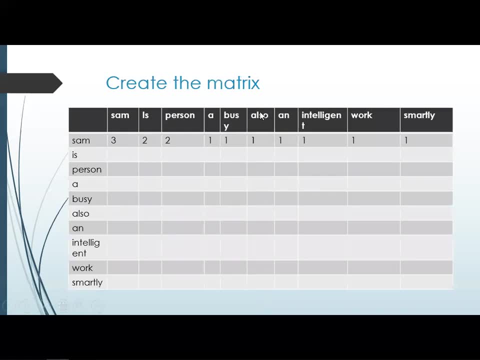 Suppose I have a sentence saying that I'm going outside right, And at that time whenever we create some matrix. so let me just give you an example of some matrix. Suppose we are creating this particular matrix, right, And I have various sentences. 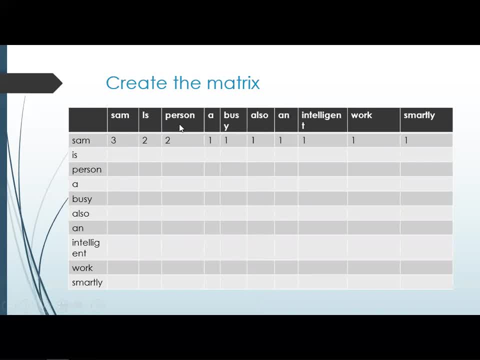 Suppose I have three to four sentences and this particular matrix. we always do not follow the order, you know, order of this particular words because in a sentences we have some order of the words Which actually indicates you know the relationship between two to three words. 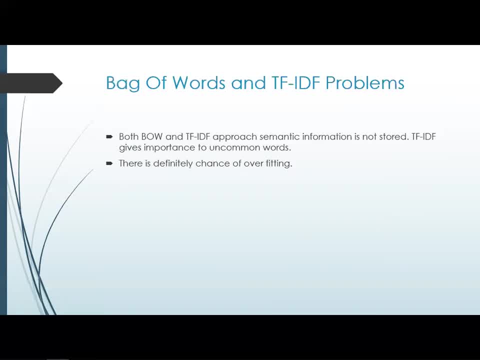 But when we are actually discussing about the problems of bag of words and TFIDF, this semantic information is not stored. That is pretty much important to understand, Okay. And when we are applying bag of words and TFIDF, there is also a chance of overfitting. 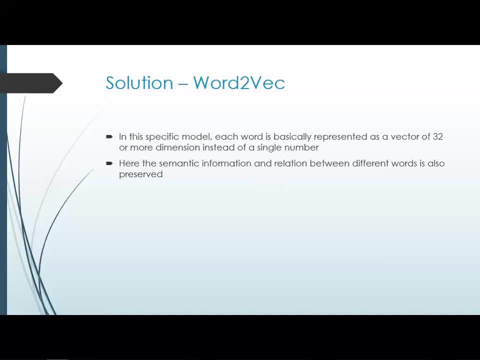 Now, in order to overcome this particular solution, what we do is that we use something called as word2vec model. Now, what exactly is word2vec that we are going to discuss? In word2vec, what we do is that each word, you know, instead of assigning values like ones or zeros, or assigning some values like 0.43 with the help of TFIDF or some other values, 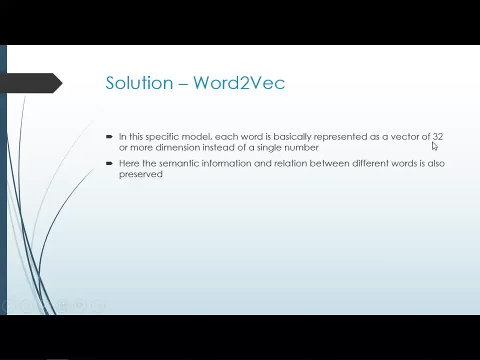 Instead, what we do is that each word is basically represented as a vector of 32 or more dimensions instead of a single number. Now you will be getting confused with this. Don't worry about that, guys. I'll be explaining you about this with the help of a practical example. 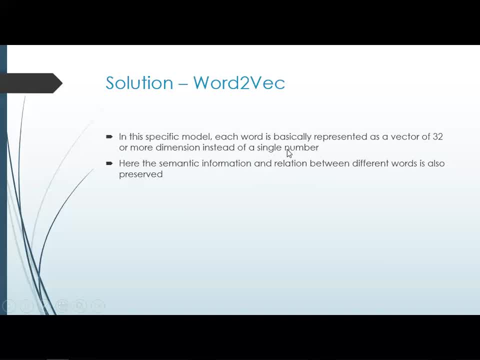 So, in short, what will happen is that each and every word Is basically converted into a vector of 32 or more dimensions. That is what word2vec actually does. you know because you you may have probably seen some representation, right. 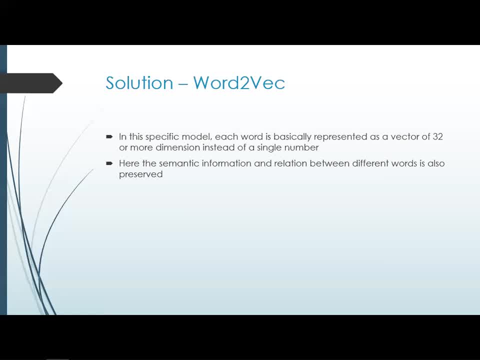 Or some representation of sentences. If you know natural language processing with the help of bag of words, we usually convert that sentences And based on that particular word, we try to convert that as one zeros And we represented that whole vector in the form of row. 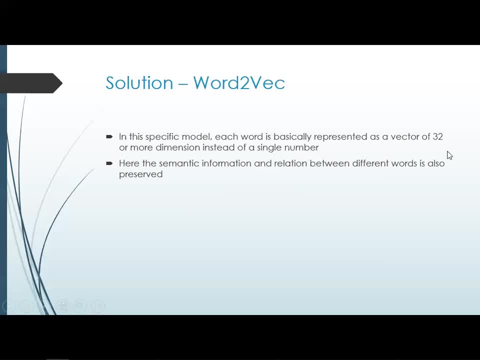 But in the case of word2vec, each and every word is represented As a vector of 32 or more dimensions. Now, because of this, what happens is that this word2vec also helps us to keep that semantic relationship, semantic information and the relationship between two different words. 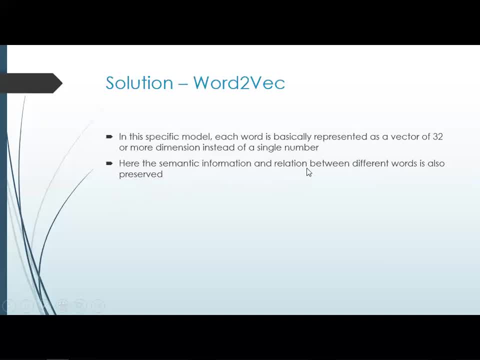 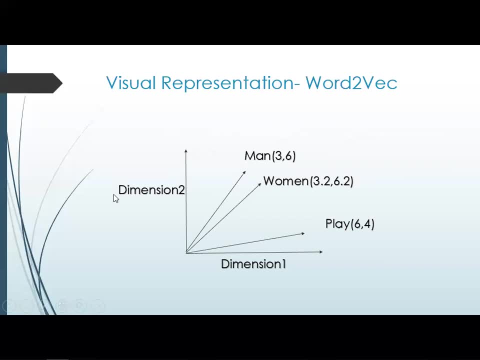 So here you can see. the second point says that here the semantic information and relation between different word is also preserved. Now you may be getting confused. Let me just show you a very good visual representation. Suppose now here. in the previous example I told you that we will be having 32 or more dimensions. 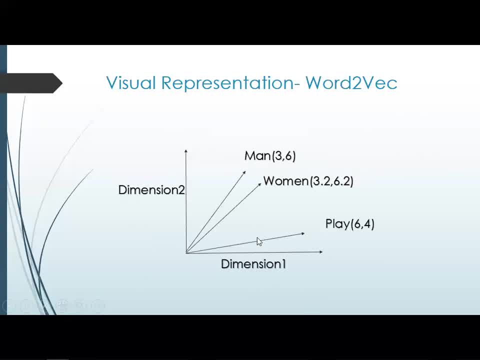 Let us just take some two-dimension example over here. what it indicates is that each and every word is represented by two dimensions, And when I say two-dimension, this, this X axis is one dimension and the Y axis is two-dimension. 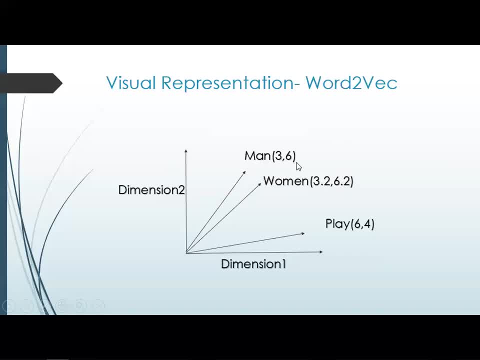 Suppose man is basically indicated by the vector three comma six. three comma six basically means the dimension one value is three. the dimension two value is six. Now, similarly, I mean now who men over here, you know that man and who men are almost similar over here. 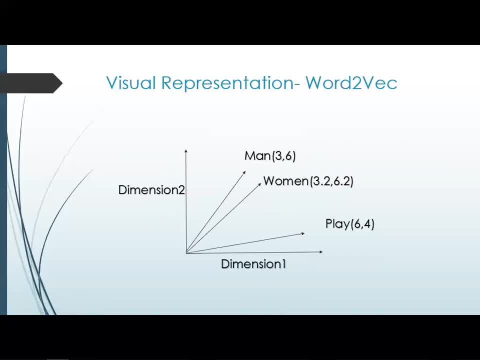 You know they are almost related, They have some semantic information, So this particular distance that you see between them should be very, very less. So suppose I have assigned a vector over here like three point two comma, six point two. So here it indicates that man, a man and woman are basically interrelated. 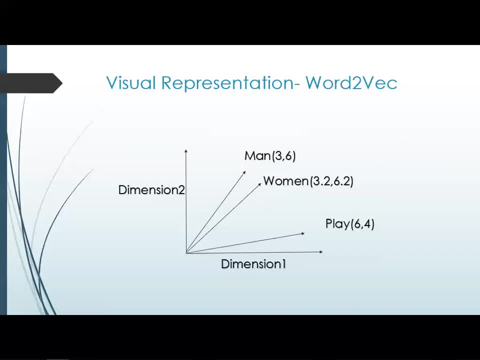 You know there is a semantic information, that is a present between them. Some some relation is there between them Now. similarly, if I take some another word like play, okay, now you can see that over here the play vector that I have- a. 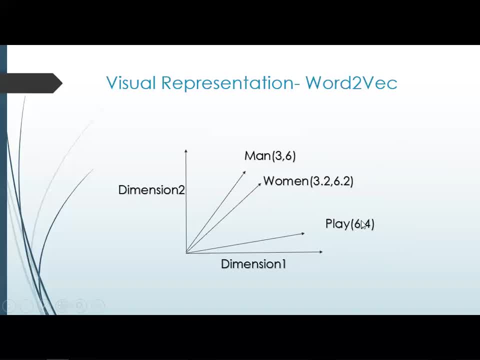 Signed a six comma four, how this vector is calculated. I'll just show you with the help of practical example, but just to understand that we are assigning some vectors of two dimensions, like dimension one and dimension two. Now over here you can see that this play may not be related to this kind of words, right? 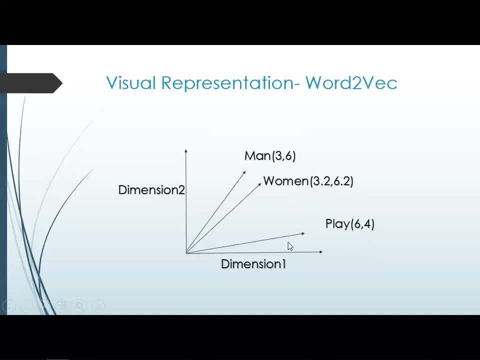 So it is present in a far distance in this particular two-dimension diagram, right? So this is how a visual representation of you know what to whack model basically looks like. each and every word over here I assigned two dimensions, So this is basically my two-dimension vectors. 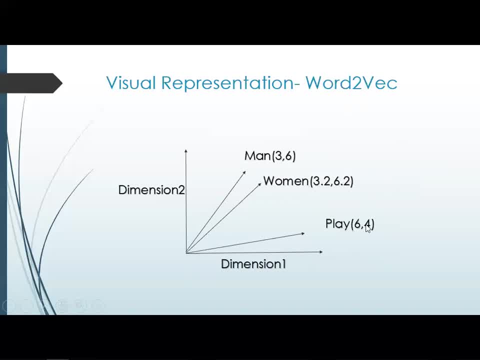 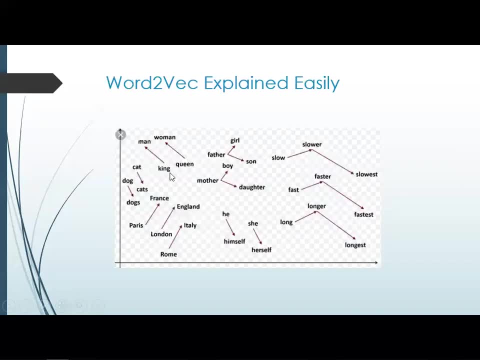 Women is assigned a two-dimension vector. Similarly, play is assigned a two-dimension vector and each and every word is assigned a two-dimension vector. More probably, if you want to see, you can see over here. you have different, different words, right. 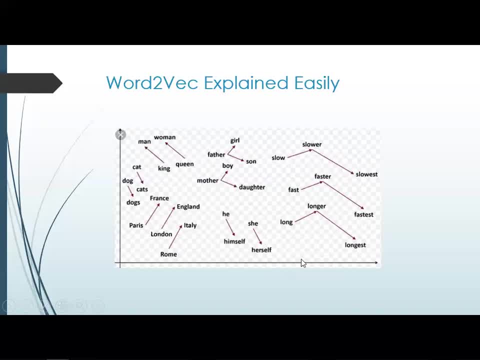 Over here you have man king. If suppose you are representing this in the form of two dimension, you can see that most similar, more common words, more interrelated words are present near to each other. The remaining words are actually far with respect to each other. right. 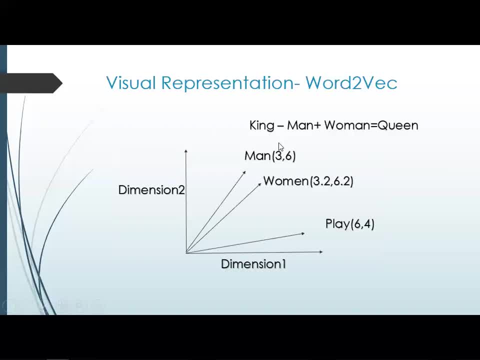 So Let us go ahead and see one more example. Now. Google is doing a lot of research in this word to work, and many companies are doing a lot of research to implement a lot of things. Now, if I have this kind of scenario and if I try to apply some mathematical equation saying that king minus man plus woman, right. 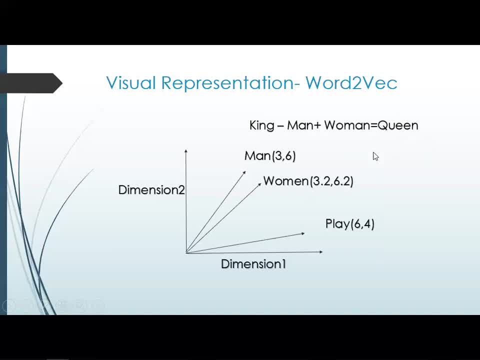 If I just try to apply this kind of operation, it will give me the answer as queen, because we know that king and queen are interrelated And if you're trying to compare with respect to a man and a woman, then definitely we'll be getting the answer as queen. 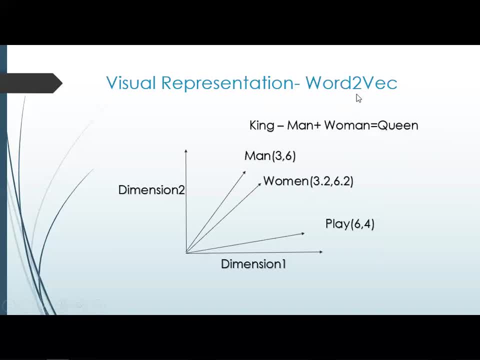 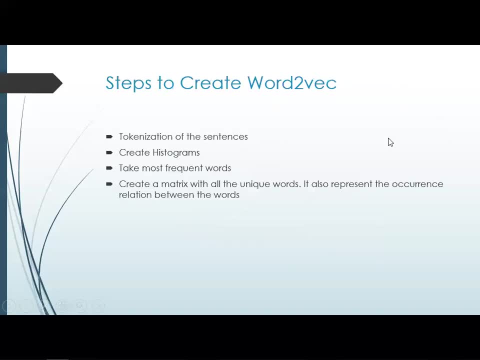 And this is accurate. This is actually true. You know, this is actually true. And this, this operation is basically taking place for the vectors, basically on the vectors itself, And hence you're getting the output. Now, the next thing is that: what are the steps to create the word to work? 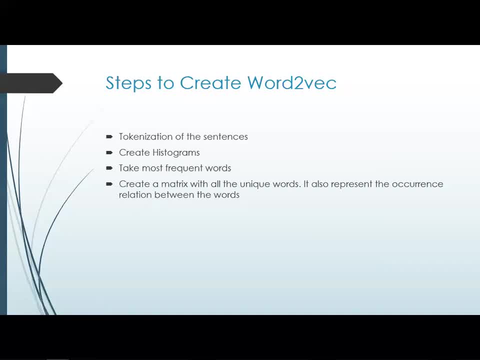 Now what I'll do is that I've written some steps over here, but don't worry about it. I'm going to show you a very good practical exam example where I'll be having a sentence and then you know I'll be doing. I'll perform some of the operations. 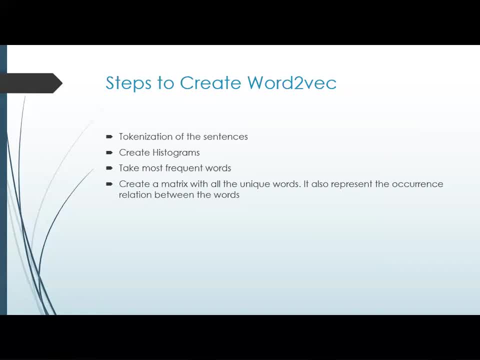 I have with the help of Jensen model. I'll convert that Into a word to work model. This lab would use Jensen library, which has this word to work, which helps you to implement, uh, whatever the word to work model that we want to basically implement. 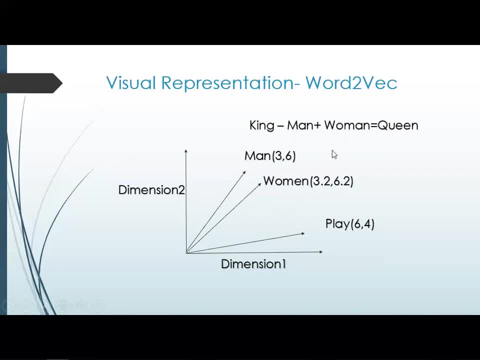 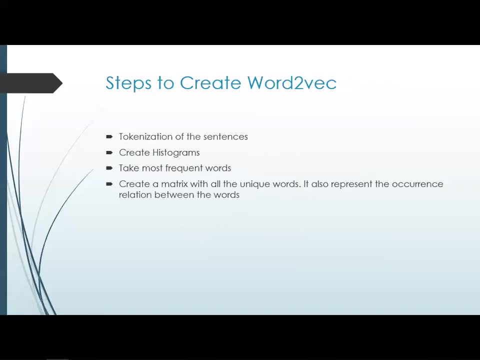 And, uh, we can assign these vectors, uh, these vectors, like how I've actually created two vectors by default, the word to work that is present in Jensen creates a hundred- uh, I mean a hundred- dimension vectors. So I'll just show you an example for that. 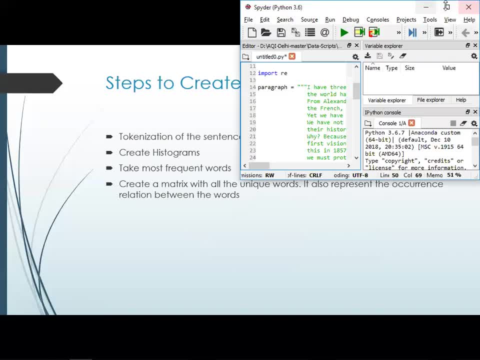 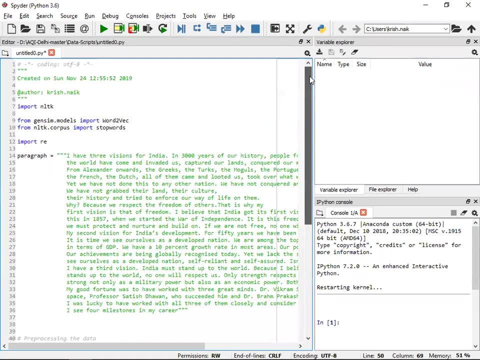 So let's go ahead and try to implement that. So here is a wonderful example. So what I'm going to do is that, first of all, I'm going to show you this particular example Now. in this example, uh, first of all you need to import some libraries. 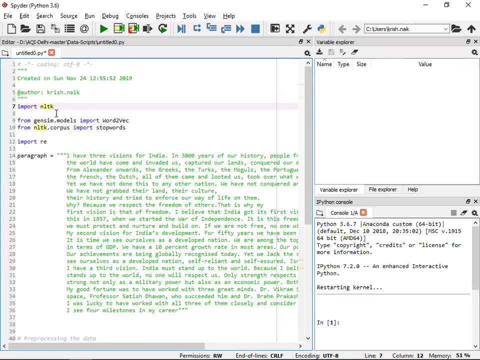 So you have an NTK library to make sure that you you install this particular analytical library. It is pretty much important because some of the functionality in an NTK, like stemming, um, you know, and applying stop keywords, are actually present over here. 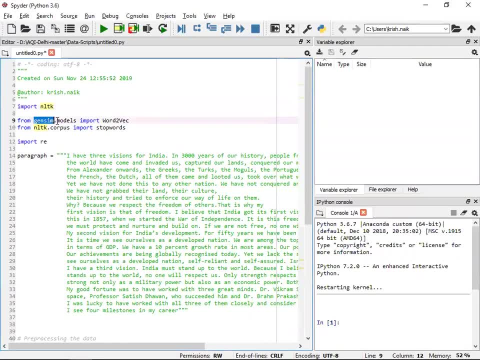 And what I'll do is that, apart from that, I'm also going to import Jensen dot models. Not this Jensen dot models, You know, has this work to work model altogether, you know, and this is already present as an open source library. 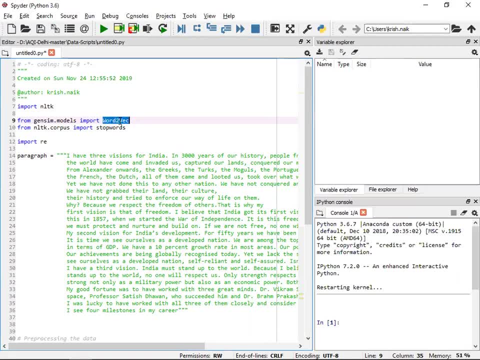 So that basically means, if I, if I give the sentences to this particular um, you know more uh- to this particular library, at that time you will be able to convert that into vectors of dimension And each and every word will be represented with the help of different, different dimensions. 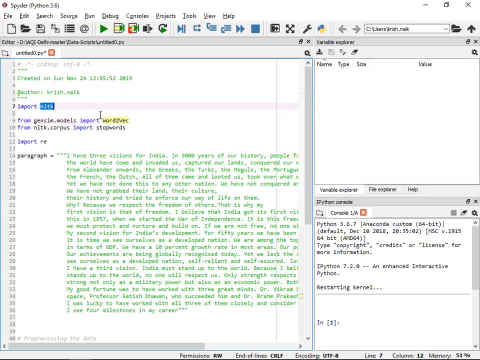 Okay. So what I'm going to do, I'm going to import an NTK, Then I'm going to import this Jensen from Jensen dot models. I'm going to import word to work. Now what will happen is that suppose this does not get executed properly. 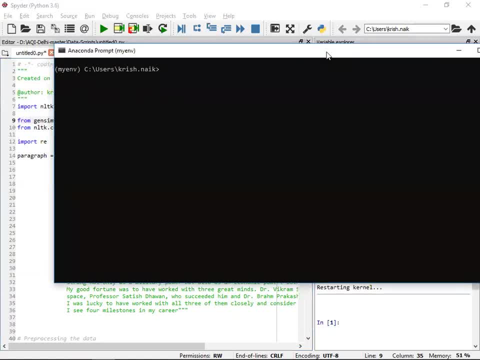 That basically means you don't have this Jensen library. So in order to install it, just go to your Anaconda prop and write pip, install Jensen. Okay, So this is what you have to basically write. It will take some time for installation over here. 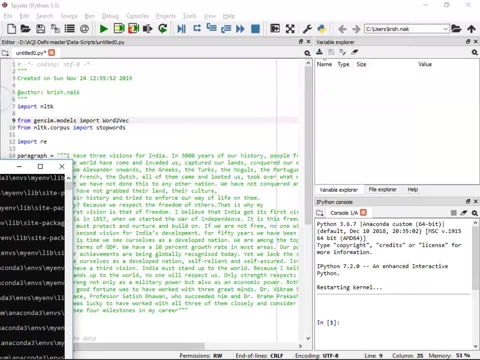 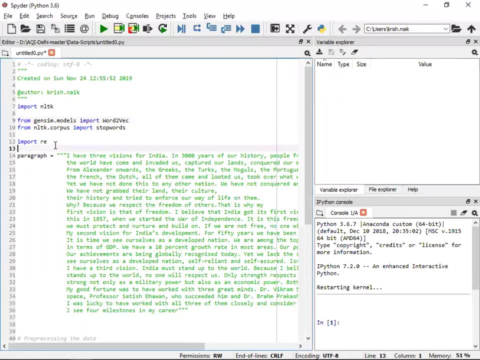 The requirement is already satisfied because I've already installed it, but it will probably take hardly 10 to 15 seconds for you to install, So make sure that you do the installation. Okay, Now I'm also going to import: Uh, regular expression. 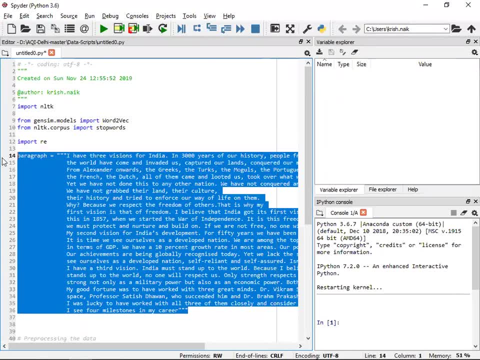 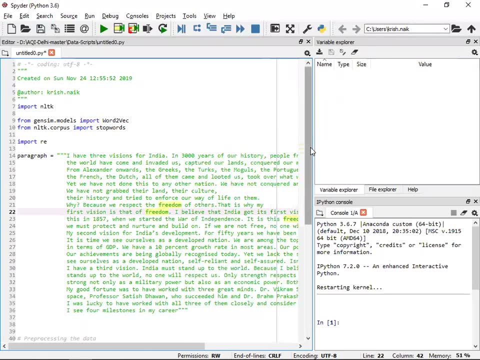 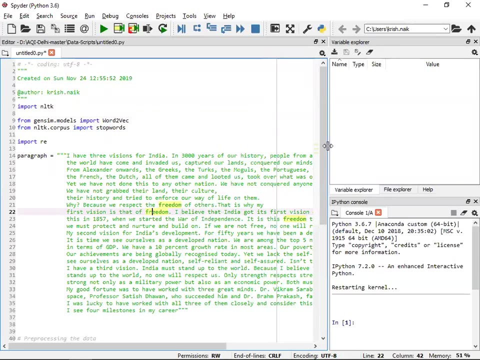 Now this particular paragraph. what I have actually taken is basically a paragraph uh of a speech of a leader whose name is, uh, APJ Abdul Kalam, And he, he was the former president of India And, apart from that, he was also the chairman in ISRO once, uh, you know, before becoming the president. 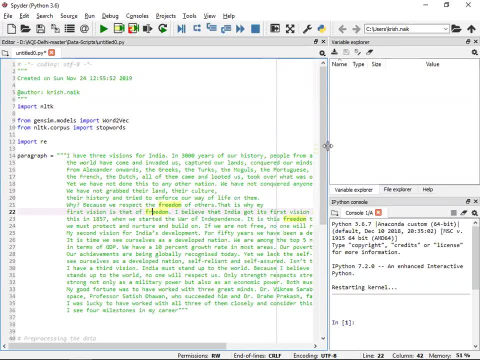 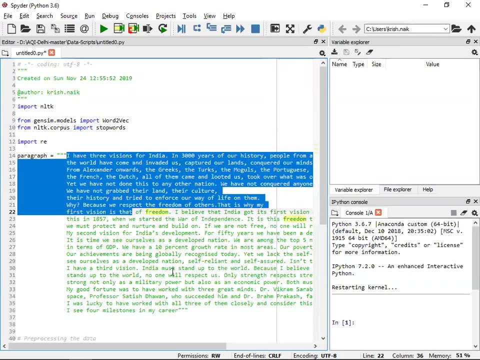 So a very good guy. Uh, I, I, I do respect him a lot, you know, for his knowledge, for his ethics, That he basically had, uh. so this is, uh, the speech of them, and this is basically a paragraph. 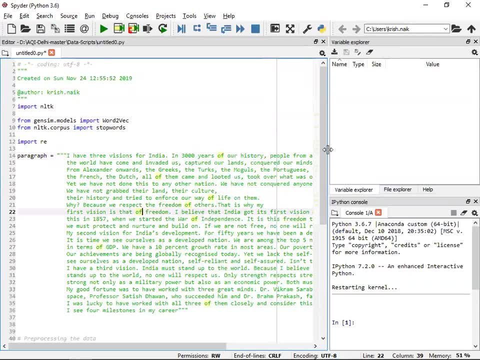 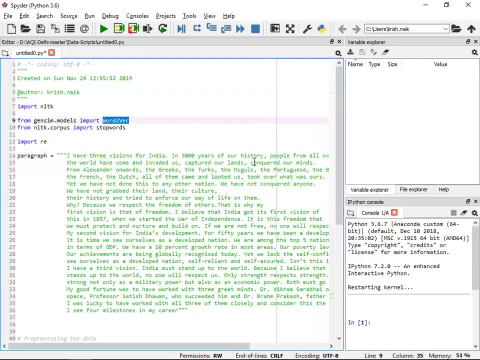 So what I'm going to do is that, first of all, I'm going to apply tokenization, because I need to convert each and every word into some vectors with the help of word to word, And that is what I'm actually trying to do over here. 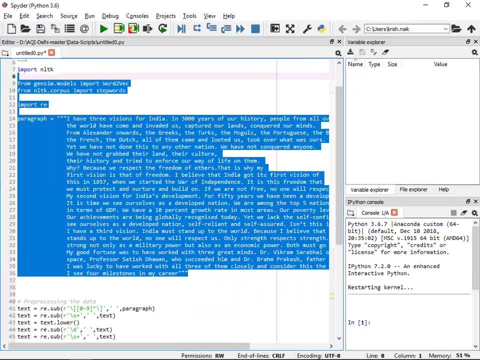 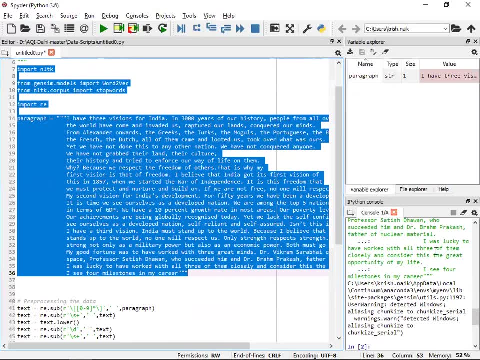 So, uh, here is it, I'm going to execute this whole thing And this, uh, this, this whole material will be given in the GitHub link, guys, You can actually download it from there. The link will be given in the description box. 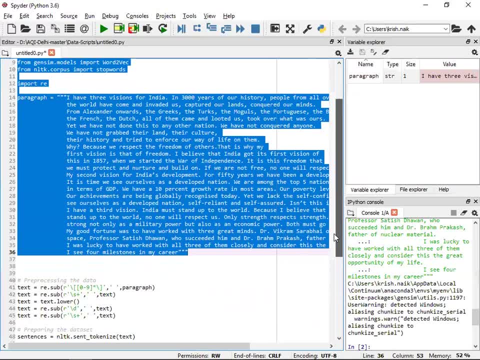 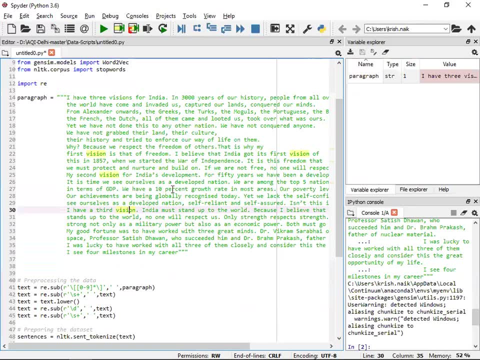 Now, After this, what I'm going to do is that I'm going to pre-process the data. Now, why I'm doing pre-processing, suppose in this particular sentence, is I have some words, I have some characters, I have some special characters. 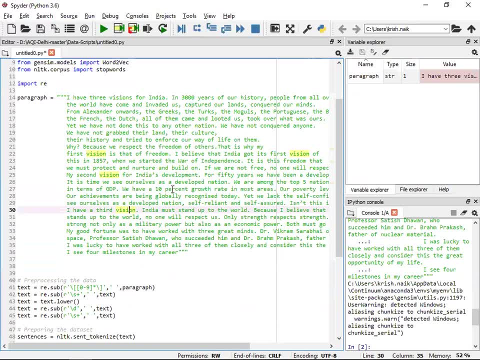 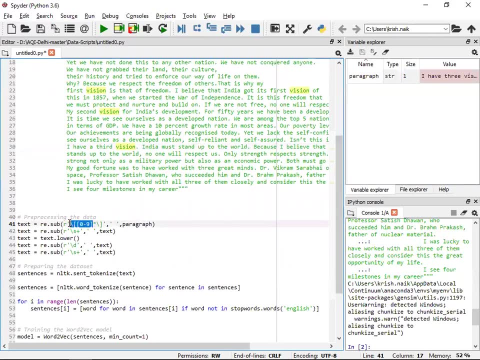 I want to remove that, you know, because that is not required, uh, in order to convert that into some vectors of dimension. So I'm basically removing all the words. I don't require it, or I'm also removing unnecessary spaces. 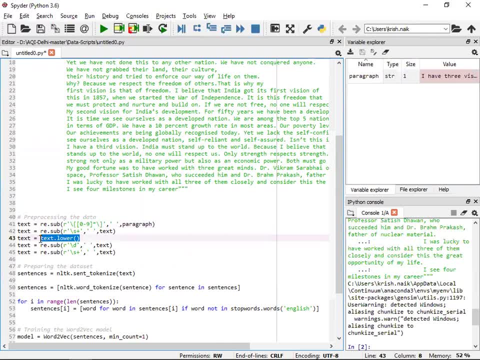 I'm making the sentences lower because the reason I'm trying to make it as lower? because, Um, you know when, when we, when we are considering as word to word, I don't want capital letters word and small letter word to be considered as a different word. 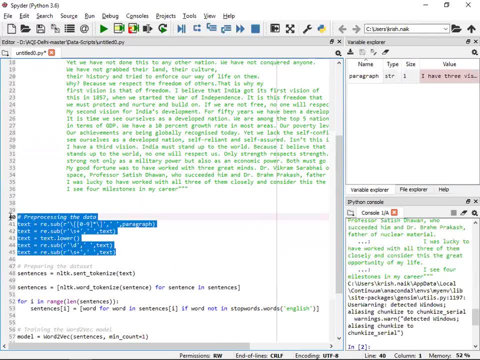 So all this particular processing I'm actually doing- and for this I'm using the regular expression- Okay, So here I'm basically removing all the words, I'm removing all the special characters and additional spaces, I'm also lowering it and I'm doing all these things. 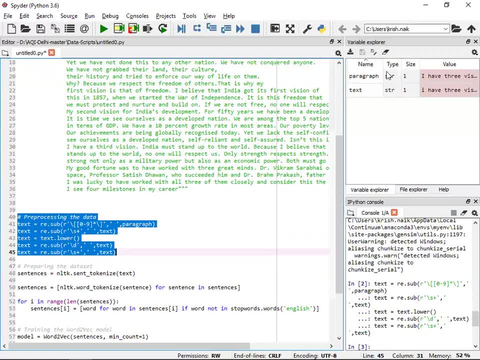 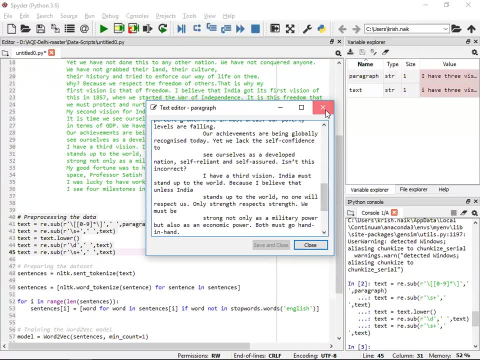 So here it is. I've got executed this perfectly. You can see that now this is my paragraph. So you can see My paragraph has many spaces over here And after I apply this pre-processing, this is my text how it looks like. 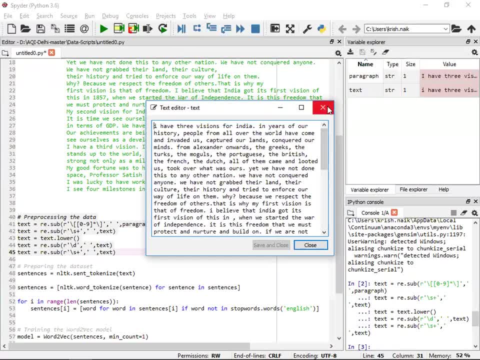 Right, And the text looks pretty much good now. Okay, Now, the next step is that what I'll do is that I'll convert this text into sentences. Okay, And in order to convert this into sentences, I have a function which is called as: NLTK dot sent underscore tokenize. 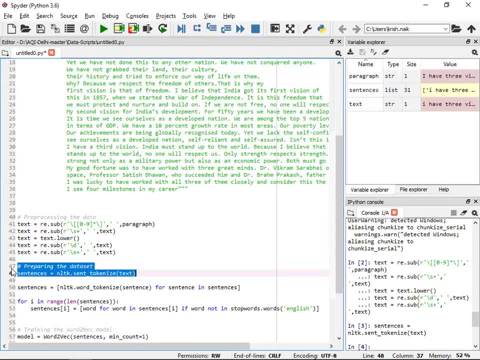 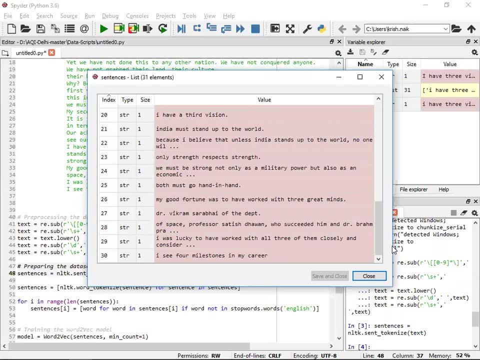 Okay, So I'll go and execute this. So as soon as I execute this, you can see that I'm getting a list of sentences over here, So 31 sentences. that basically means that paragraph has got converted into sentences. Okay, So pretty much simple. 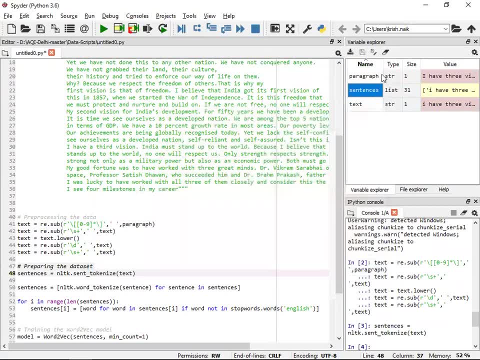 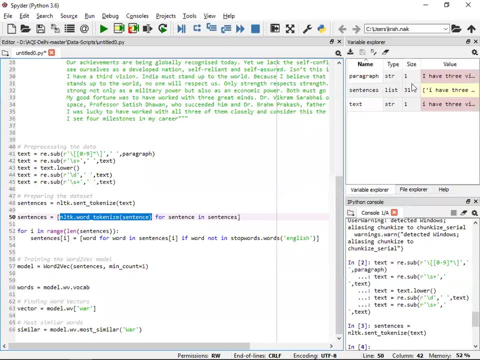 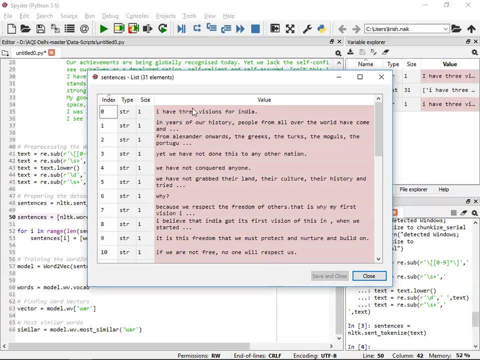 This is. this process is also called as tokenization. Okay, So this is pretty much important. Now, what I'm doing over here is that I've used a list comprehension, and now, for each and every sentence that I that is present over here, I'm going to convert this into words, you know. so I'll just write: I have three visions. 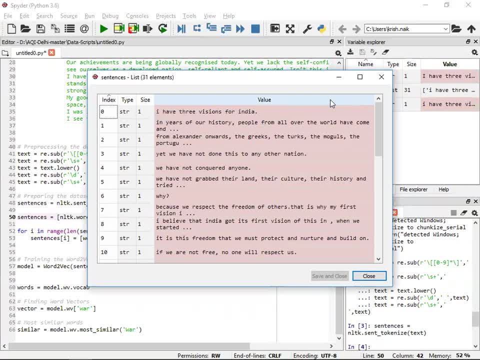 So all I'm doing is that I'm trying to convert this into words. The reason I'm trying to convert into the this into words? because they are some, some words like we, the of, if, he, she, so this kind of words are basically called as stop words, you know, and they are present a lot of time, you know, so we should try to remove it, and that that can be removed with the help of stop words, a library that is basically present in NLTK. 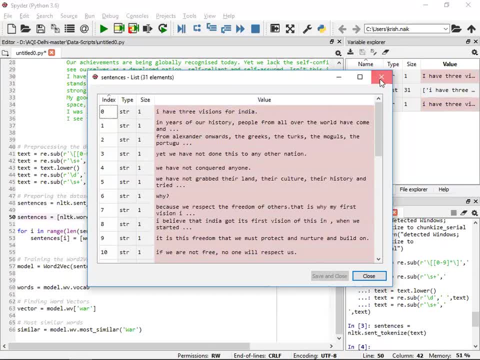 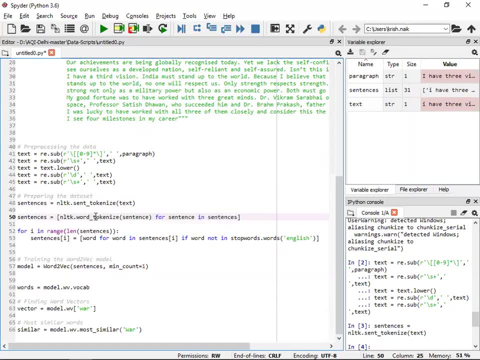 So I'll just show you how to do that, But what I'm doing currently over here. first of all, I'll convert all these particular sentences into words. So I'm using a list comprehension saying that NLTK dot word took an eye. 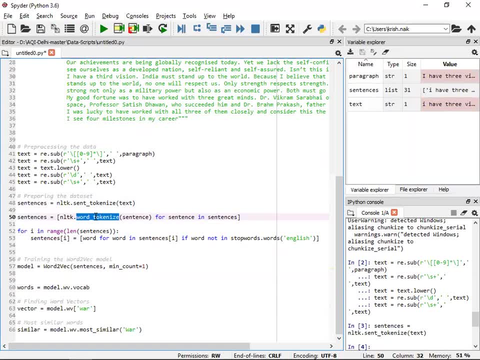 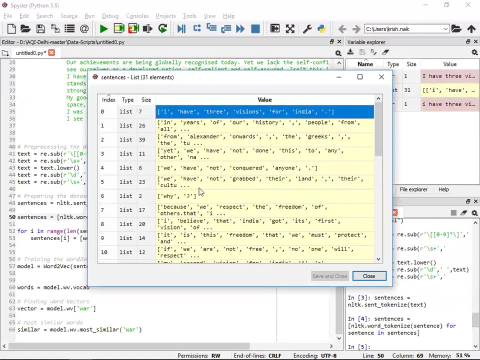 So this is the function which will convert all the sentences into words for sentence in sentences is I'm looping through all the sentences and it will finally convert this into words. So once I execute it now, you can see that I'm having all this particular words over here for all the sentences. right now, each and every sentence has got converted. 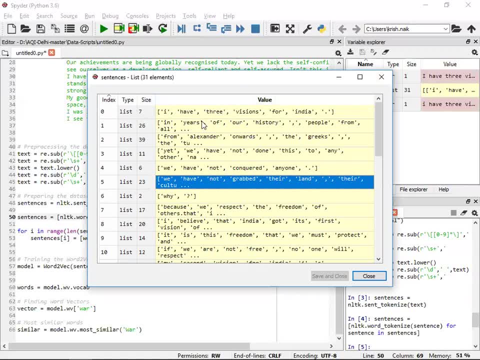 Now, what I'm going to do is that I'm going to again loop through all this particular thing and I'm going to remove the stop words like for if I have she, he, because I don't require that particular word, because those will be present many number of times. 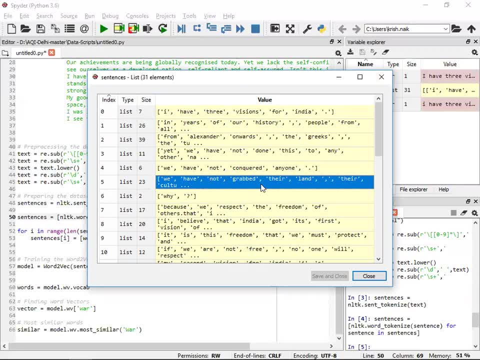 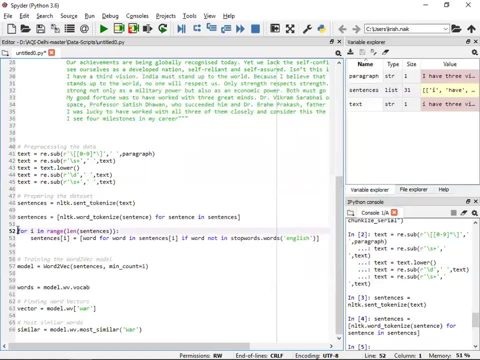 And usually for spam classifier. for for most of the scenarios, I don't require this kind of work. So what I'm going to do is that I am going to put a for loop. So this for loop actually helps me to you know. remove the stop words. 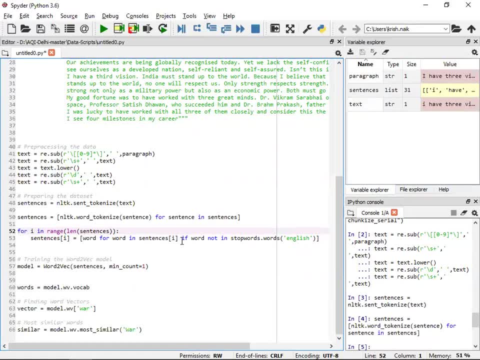 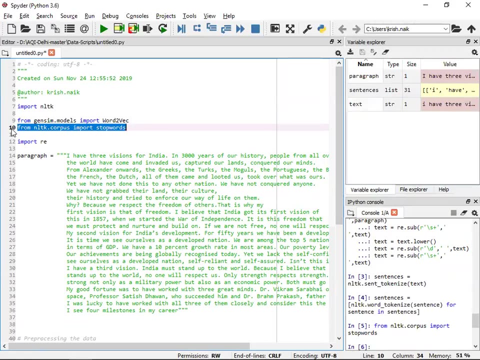 You can see that I've written word for word in sentences of I if word, not in stop words, dot words of English. Now, if I Just execute this, before executing this, I hope I have executed this particular library, because this particular library will help you to download the stop words. 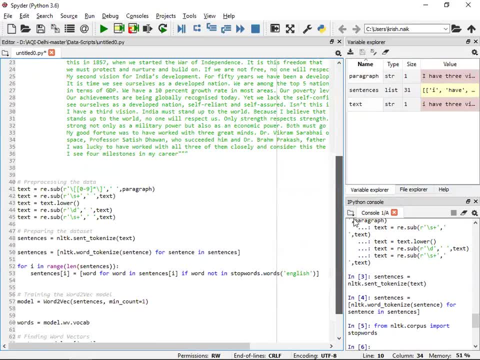 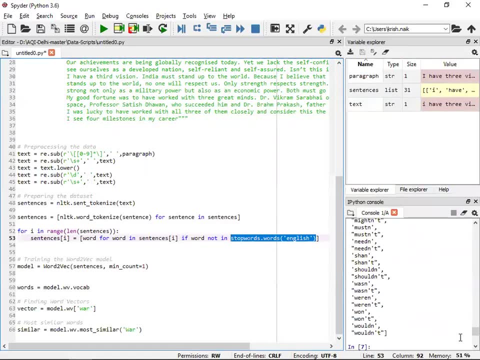 Okay, So, um, here it is, And what I'm going to do is that I'm going to execute this stop words, dot words of English. This will actually give me all the stop words that are present in English language. You can also store this in the. uh, I'll just execute it, just second days. 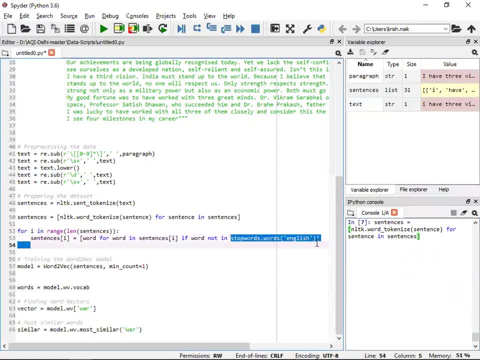 I'll just execute it once more So that I see all the stop words. Okay, Now you here, you can see all the stop words that are present in English language. What you can also do is that you can also save this in one variable, and then you know you will be able to execute it. 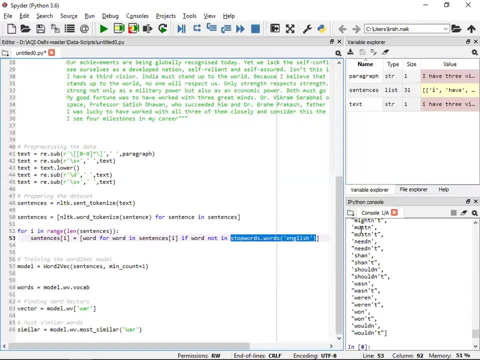 Okay, Uh, you can store it in a variable, then apply some conditions and then you try to remove the stop. That is also possible. but understand this. this is again a list, comprehension. What I'm doing is that for every word in sentences of I- because I'm actually looking through all the sentences- 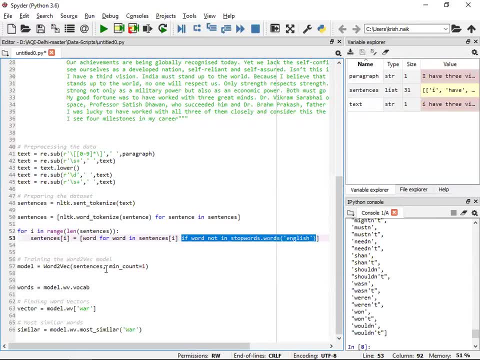 I'm saying that If the word is not present in stop words dot word of English, I'm going to just put that particular word only in the sentences. Other than that, I'll. I'm just going to remove it, So once I execute it. okay. 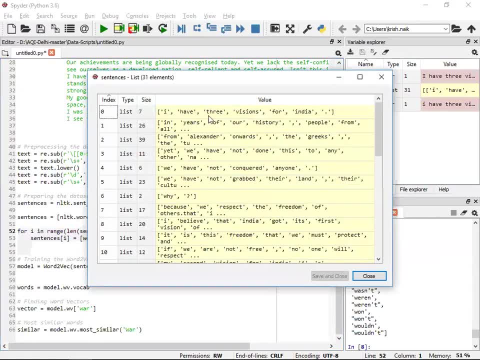 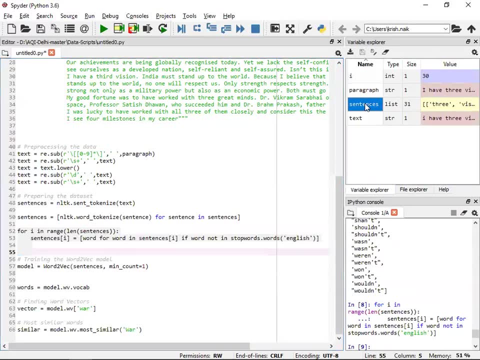 So here you can see initially my sentences is having. I have three vision for India. Now what will happen once I execute this particular sentence? So here it is. You can see that now I have all got removed, because those who are basically stop words. 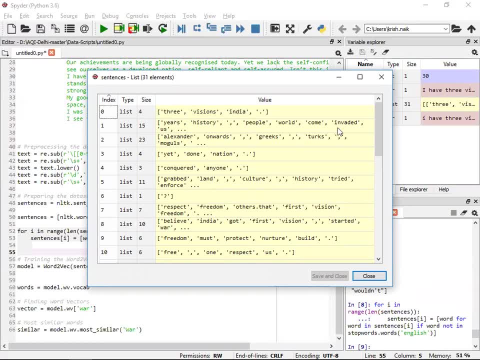 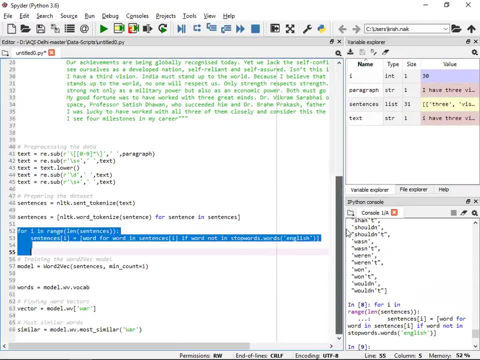 Now I have three visions. Then the uh years, This three people will come, invaded us. So all these kinds of word are there, Okay. Now the next thing is that I will try to apply my word to where. now, word to where is a pretty much popular library. 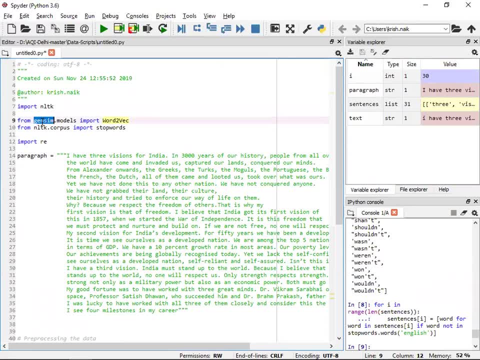 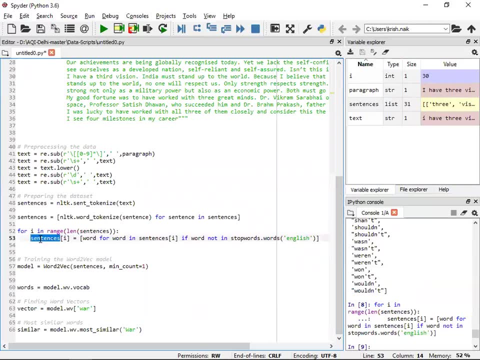 The word to where library that I'm going to use is something called as Jensen. Okay, Now, this particular library. what I can do is that I can pass this whole sentences. Okay, Whatever sentences I have generated, I'm going to pass this as my first parameter. 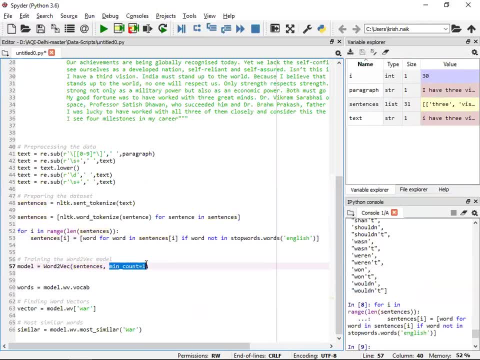 The second parameter basically says that Min underscore count is equal to one. that basically indicates that if the word is present less than one, then I am going to just skip that particular word. But if a word is actually present, I usually have at least one count. 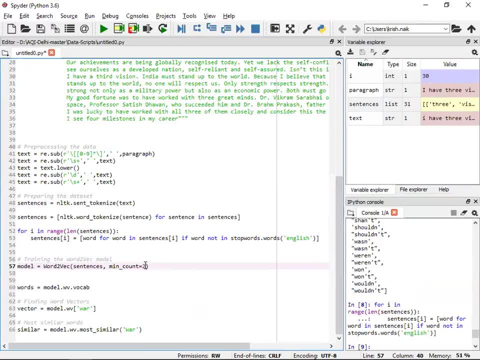 So usually people, what they do is that they they try to put this number as two, which says that if the word is not present more than two times, if it is present less than two times, just remove it. You can also play with other the values like five. right now my data is very, very small, uh, because word to work is applied for huge amount of. 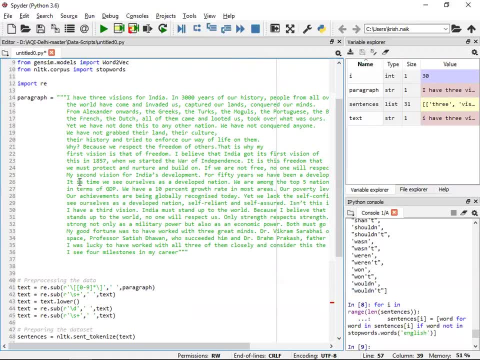 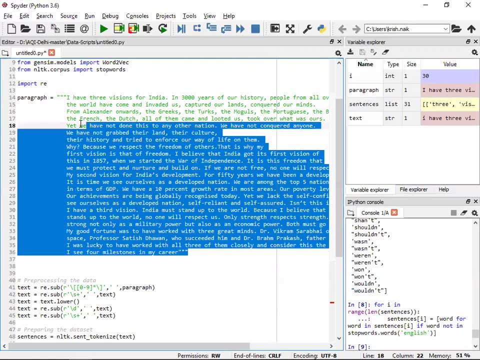 Data like from from: uh, we may basically take the course from the whole Wikipedia and then you can apply word to work to get a better result. But just here I want to show you a very good example, So I've taken this particular paragraph. 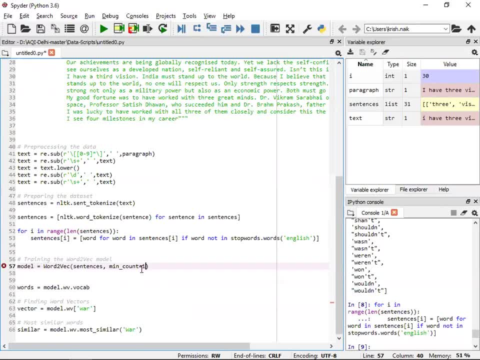 So what I'm going to do over here? I'm just going to make this min count as one. Okay, I'm going to execute it Now. you'll be shocked to see that it has got executed so quickly. Right, But understand, guys, this is got executed very quickly because the data is very, very less. 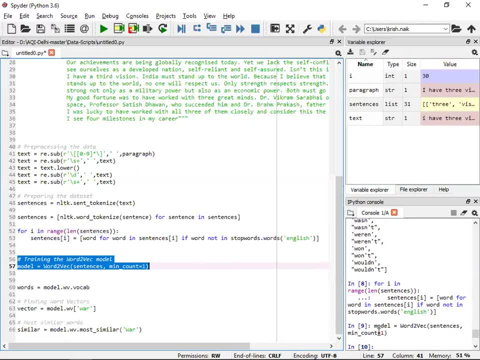 If the data was huge, it will definitely. It will take more amount of time, you know, to execute it. Now what I'm going to do is that, as soon as I executed this, I will go and find out the vocabularies that have been found out in this particular word: to work model. 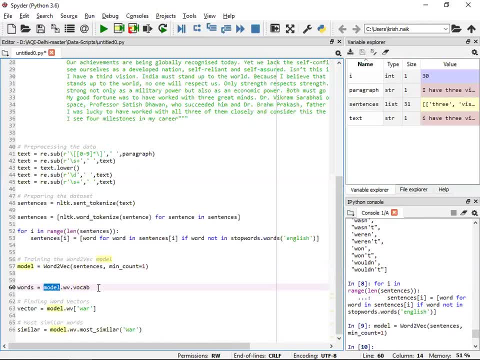 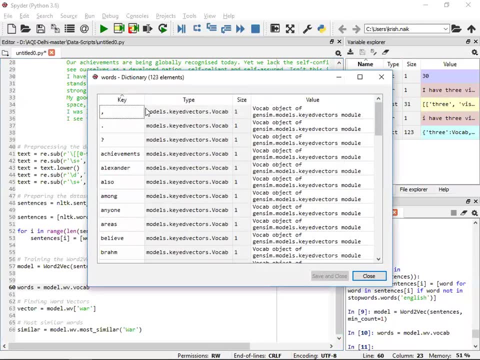 So for that I'll just execute modelwvvocab and I will store it in a variable called as words. So once I do this here you can see my words are basically all these things: achievements, Alexander, also among anyone. So this will actually be shown in the form of ascending order with respect to alphabets. 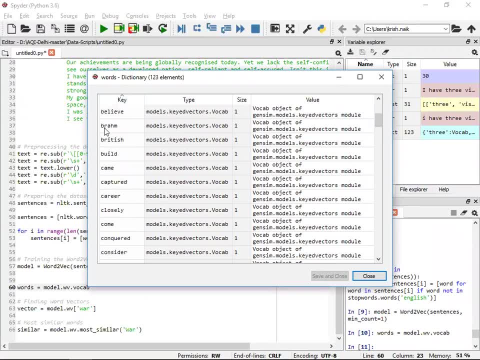 And here are all the words that we can actually see, And for each and every word there will be some you know, some, some some vectors, dimensions, pieces. for those you know, it'll be represented with respect to vectors of hundred dimensions. 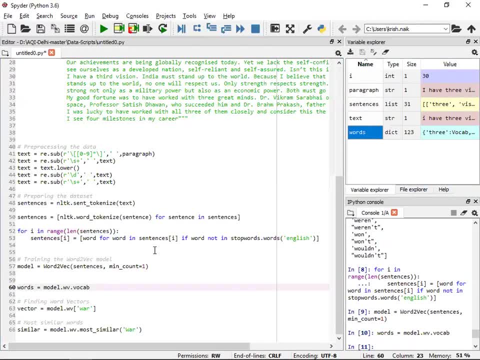 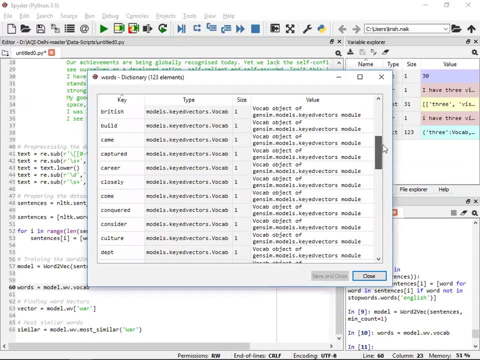 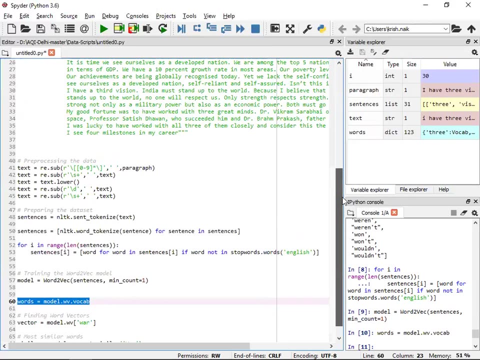 What I think for with respect to this. Okay, So it will be having vectors of, um, you know, a hundred dimensions in shot. So, uh, yes, Uh, so This is, this is the type of vocabulary that we are basically getting now. apart from that, what you, what we can also do, is that suppose? uh, let me consider it. 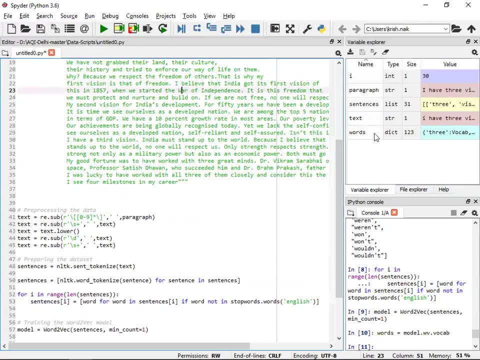 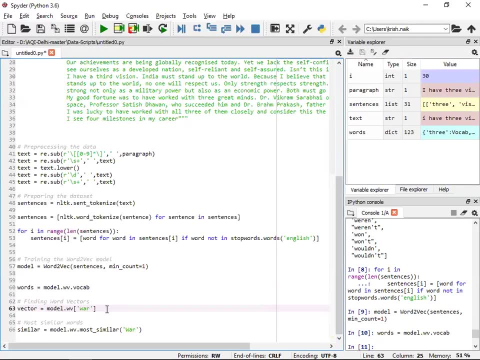 There is a word called as war. Okay, Now, if I want to find out the vectors and if I want to see the relationship, what I'll do is that I'll just write modelmv of- uh sorry, modelwv of war. 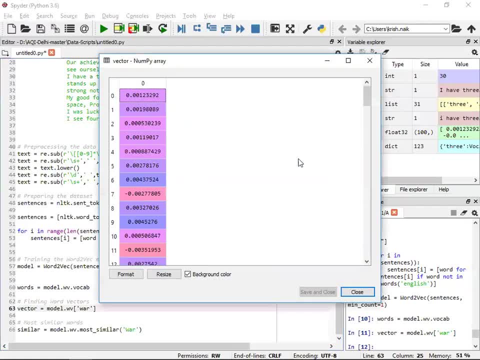 And I will try to see the vectors. Now, if I go and see the vectors, this is basically the vectors of that particular word: war. you know, this is the vector Of that particular word and war and you can see that it is having a hundred dimensions. you know a hundred dimensions. 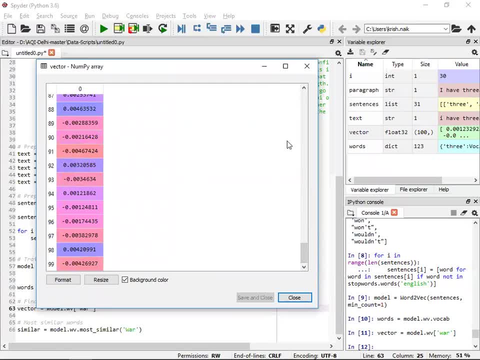 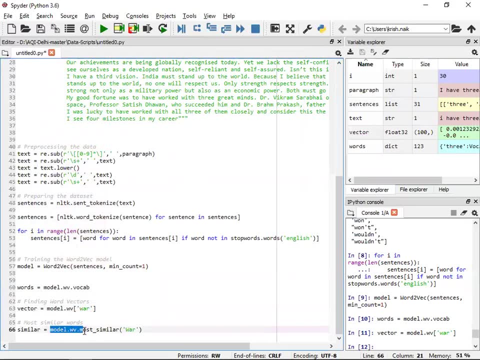 So this is what it is basically representing. Now, if you want to find out the similar words with respect to war, how do we find out? So I'll be using the same modelmv and there is a function which is called as most underscore similar. 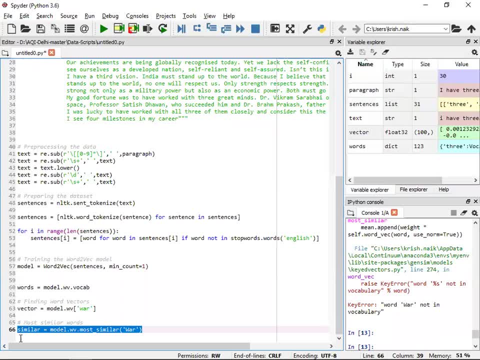 Now when I put most underscore similar of war here inside the similar variable, I'll be getting all the particular words. Okay, I'll make it that small character because I don't have any capital letter over there, But now I'll try to find out the most similar words. 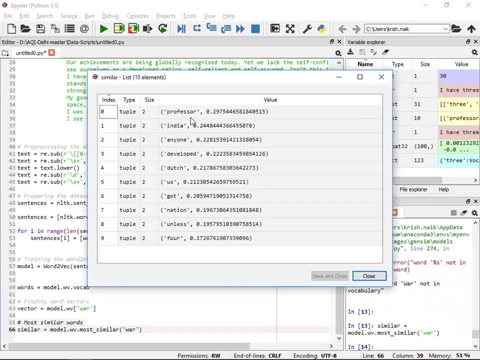 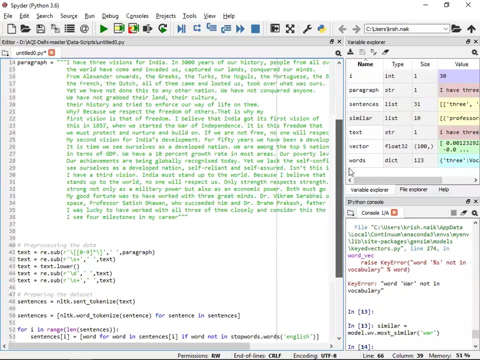 So here it is very much easy If whenever I have war, war there are similar words like: professor, India, right, Anyone developed Dutch, us got nation unless for. so it is basically showing this all things, And this is based on this particular sentence, guys. 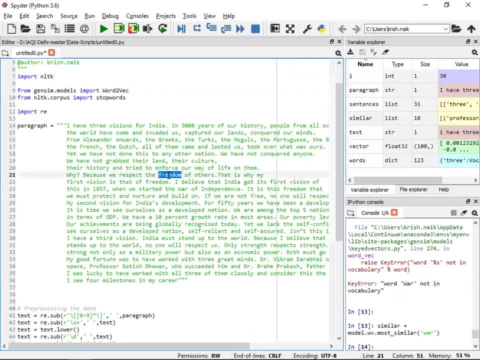 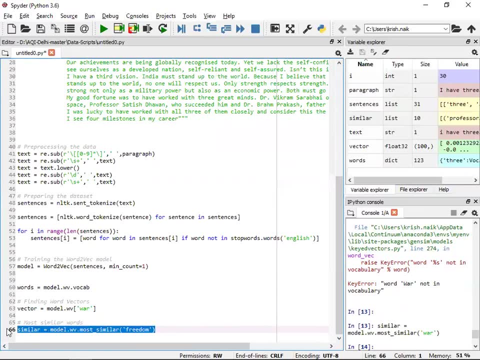 Okay, This is based on this particular sentence. Suppose, if I take an example of freedom, okay, If I, if I just go and put the most similar, I want to find out the Most similar word with respect to freedom. Okay, 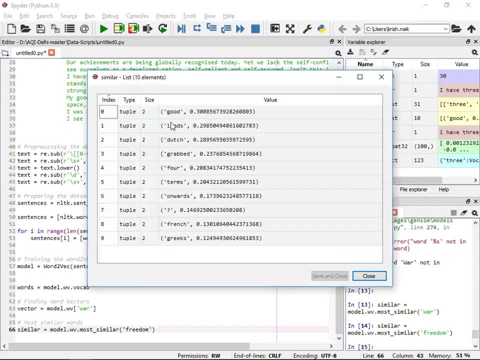 Now, once I execute it. now, if I go and see my similar metrics, you can see that freedom, good lands, Dutch, grab four terms onwards: French, Greeks. It is finding this most common words because, uh, in that particular speed, they have talked about the freedom fighters with their talk about, uh, you know, uh, independence. 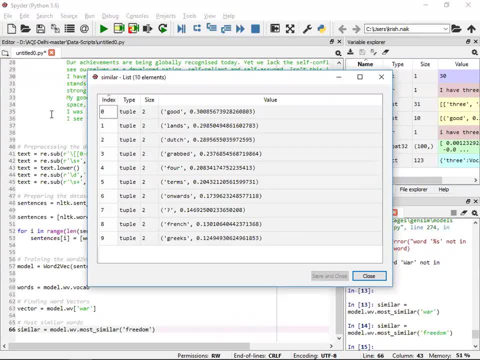 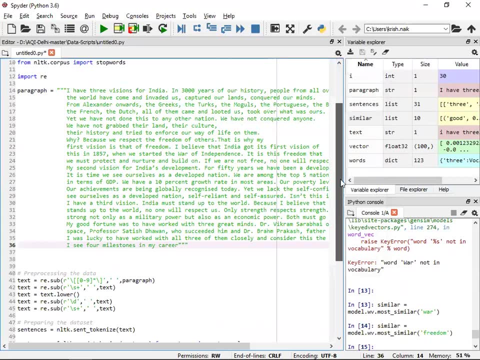 They have talked about uh, different, different uh related to independence itself, uh, and all the achievements that basically India has actually done. So This is pretty much important that you can also find out anything, anything Basically you can. you can take like this name also for that. 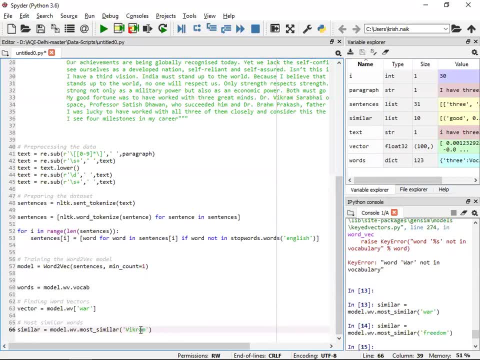 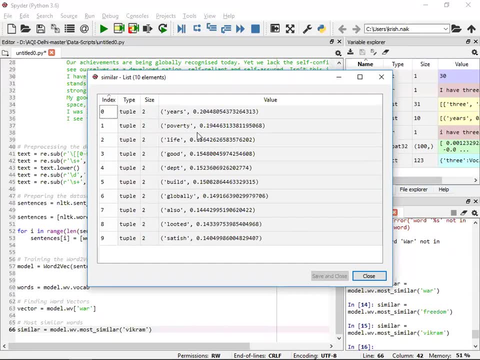 They can victim over here, And Vikram Sarabhai is also a very popular person. So if I, if I execute this and if I go and see my similar things now, you can see that, with respect to this particular word, you have yours. 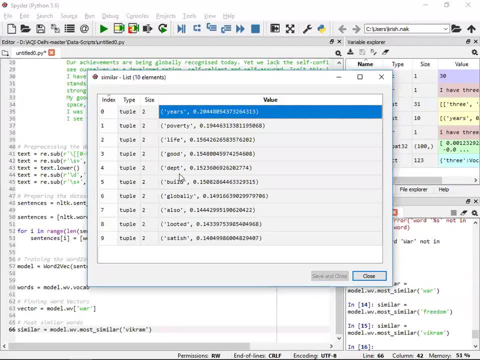 And these are the most common words, which is basically in that a hundred dimension. you'll be seeing that this, this, this, this, this, uh words will be pretty much near to This word that is victim, Okay And uh, this is what. and from this you can also see that it looks very good. 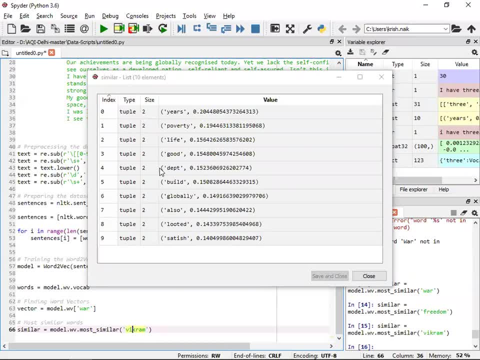 Right, And just with the help of this many sentences we are able to find out the most similar words very quickly. Now just imagine, guys, if our data set is very, very huge, a huge amount of data is basically present, Then what will happen? 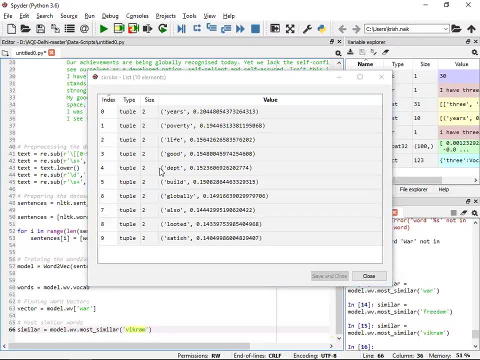 You know there's a whole lot of scope of what do we can. still more research is basically going on. They are even work to work that are given by Google itself and it is available, Uh, in the internet as an open source. on the you can directly upload that word to work and you just have to give those sentences and automatically they'll convert this into vectors of dimensions. 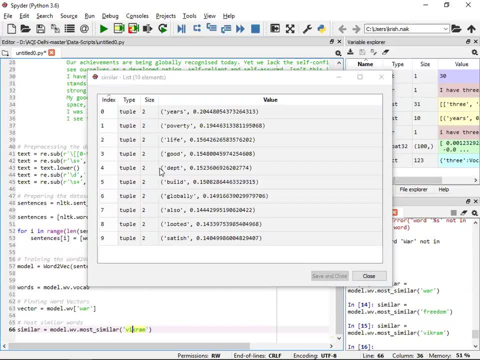 And, uh, I've worked with one Google word to work. uh, you know, if I let me go and search in the Google, you'll be able to find it also. So, yes, uh, this is an example of what to work. 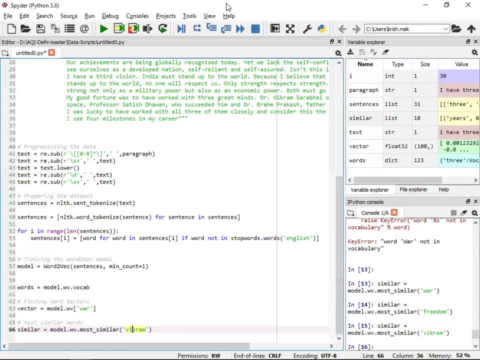 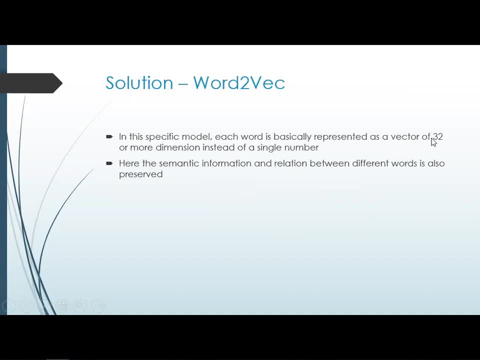 The main thing is that you are able to find out what what we are trying to do with work. Let me just go back over here. in this specific model, Each word is basically Represented as a vector of 32 or more dimension. 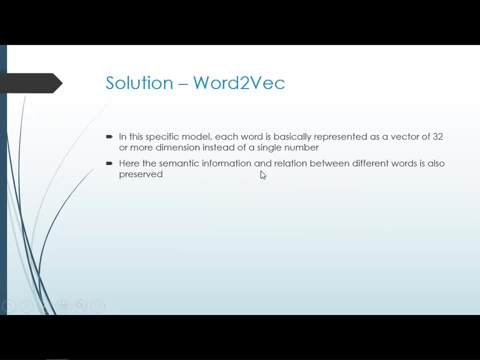 In our case, we have a hundred dimension here. the semantic information and relationship between the different word is also preserved. This is the most important thing, because this was a problem with respect to bag of words And this was a problem with respect to TF idea. 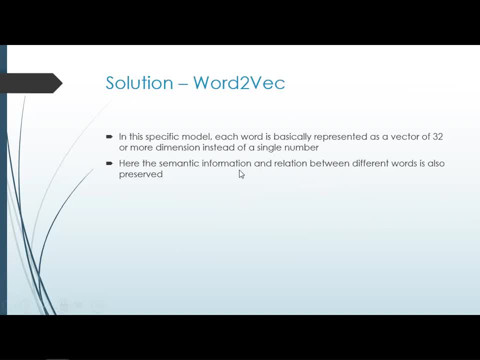 The semantic information was not stored. Uh, and if I just talk about TF idea, they used to give importance to some uncommon words. If you don't know about TF idea, Please go and visit my NLP playlist. The link is given in the description. 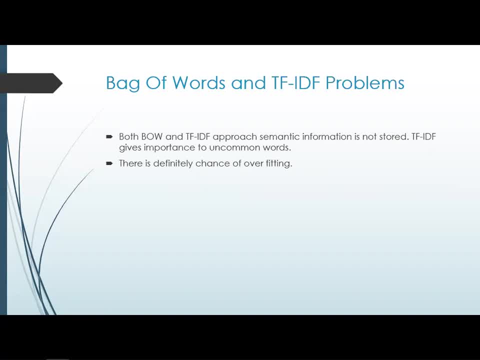 So so, yes, uh, now that if you're looking for some transition towards data science from leading data scientists to people who are working in real world IT industry related to data science projects, please make sure that you watch the YouTube channel of springboard India and that they have a whole lot of videos. 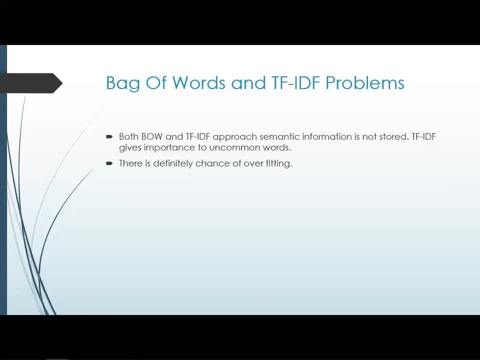 The link is basically given in the description And, yes, this was all about this particular video. Please do subscribe the channel If you're not already subscribed. I'll see you all in the next video. Have a great day, Thank you.